Yeah, guys, we should have recorded a long time ago. So, basically, as we discussed, when we're doing the vector algebra, the x-axis is on the top right. The x1 is on the top, So this is x and this is y. So we know that x runs from either left to right or right, or right to left right. 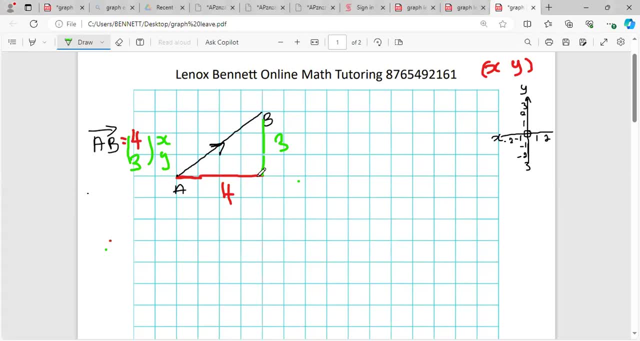 So, like our positive, are we going to our right? That would be positive. 4. In this case, now we're going up, Just like with the Cartesian plane, as I show you guys here. if you're going up, it's going to be positive, And then you just simply say how many places you. 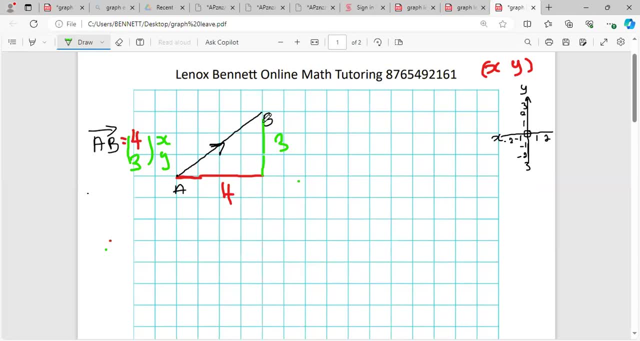 move up, And in this case it was 3.. So that's the vector 4, 3.. So you see, it doesn't necessarily have numbers on it for you to have the vector. Now, if we look at our next one, just for more, 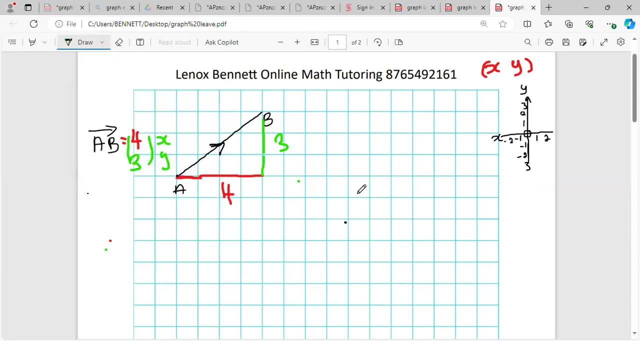 clarity, because one example: now I'll go really Get it. So I'm going to see if we can see get it further. I'll try to draw that one as straight as possible. All right, I'm going to call this one cd. So we want to name this vector. 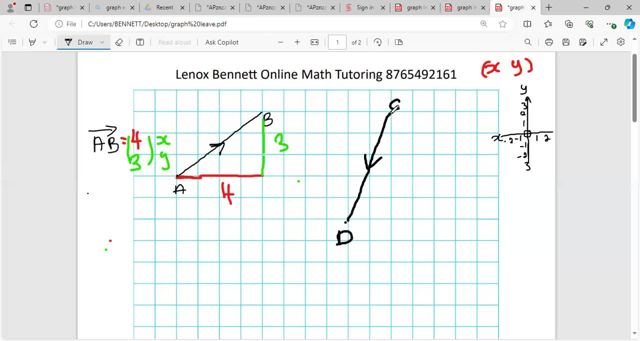 As I said, guys, you just observe the start point. You can know the start point because you see the nth, The nth, The nth point, that's where the arrow is pointing up. so we know, so we end at d because the arrow is pointing. 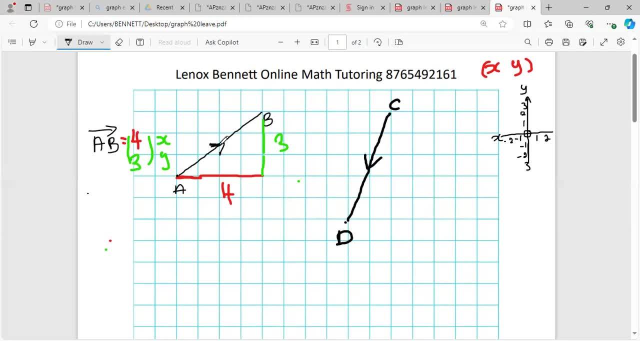 at d, just like in this case, where the arrow was pointing at d. that's our end point. so this is our end. you guys have this in your notes. so this is your start. so that's all you know. whichever the arrow is pointing to, that's your endpoint. so that means this vector is going from c to d. agree, it's. 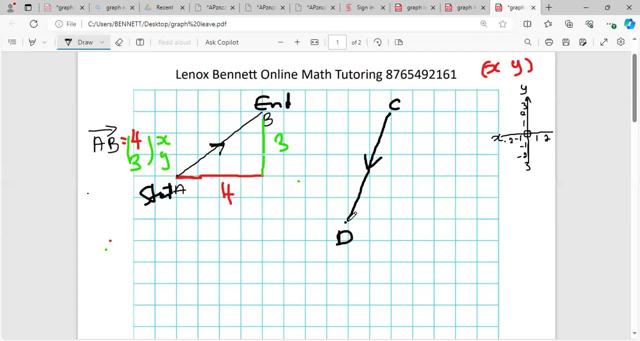 going from c to d because d is your endpoint. whichever the way the arrow is pointing, that's the endpoint. so that means this is our starting point. remember we cannot go down first. we always have to move either left or right, or the x-axis come first. so that means: because the endpoint. 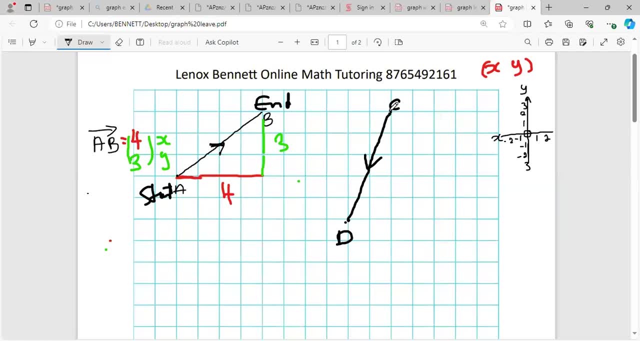 is located to the left. it means that we simply have to go that way. let me change the color so we can just kind of highlight what about. so basically now we move one, two, so we move two places, but guess what? it's to our left. so we know that on the cartesian plane, if we move to our left, 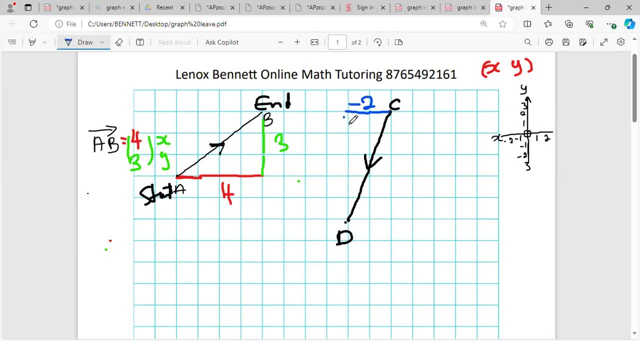 that's negative. and then now we're gonna go down, so let me just change the color again just to highlight something kind of important. and then you say one, two, three, four, five. so we're going down, guys, and this, whenever you're going down, it's negative. so this the vector that would 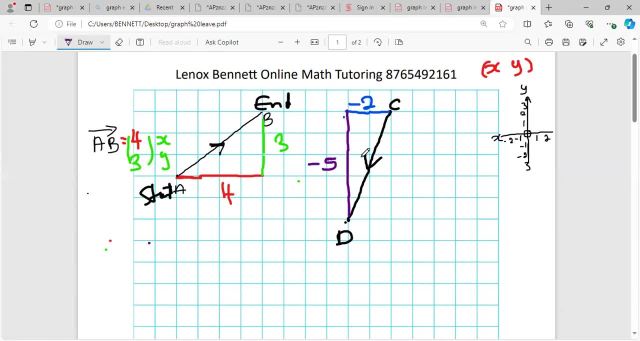 be negative five. correct, because we're going down on the y-axis. all right, sir, why didn't you go to the left? no man, if you're going to the left, that the x is negative, but when you're going down, y is negative. all right. for those who join late, let me just show you something. 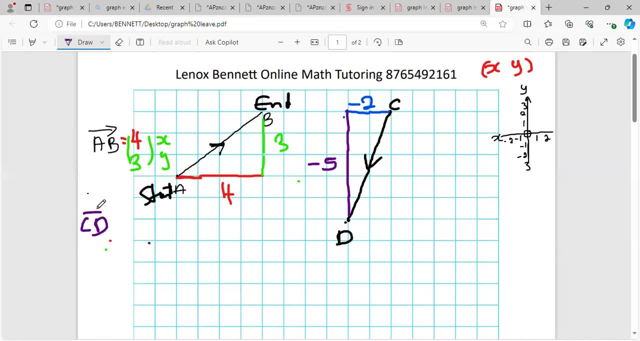 all right, guys, as i say, it can be so easy or it can be so frustrating. so in this case, that one is negative three negative five. could let him in the meeting, the john hall, if you could let him in the meeting? yeah, you see, negative three are negative two, two, two, sorry, sorry, my apologies, because it's two places to move. 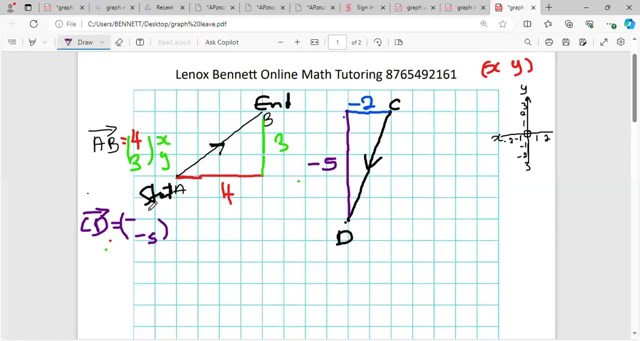 right one. oh see, two directions, i'm not sure, not sure where i treat. yeah, guys, so it's the number of places we move to our left and to our right, that's what determine the vector. i could open another scenario. so basically these are two: positive because we're moving to our right. now we're going up, right. 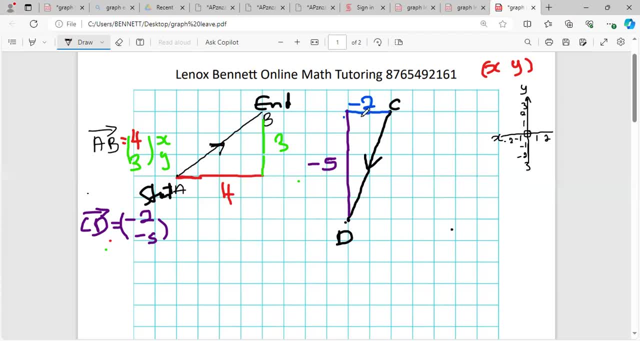 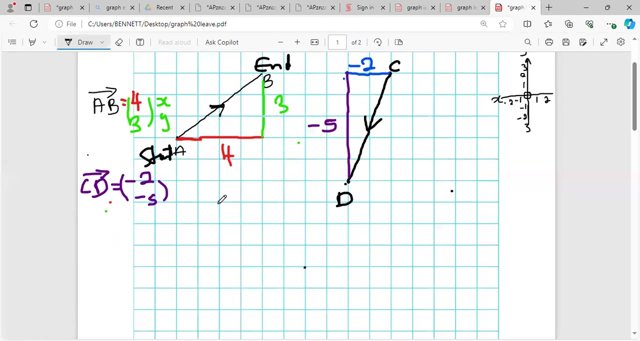 this one, we're going to our left and then we're going down. look we do another one and i basically want to capture all the possible scenarios. so let's say one point that this neighbor command and this neighbor i want to be sure i keep everything right. all right, look what happens in the next states. 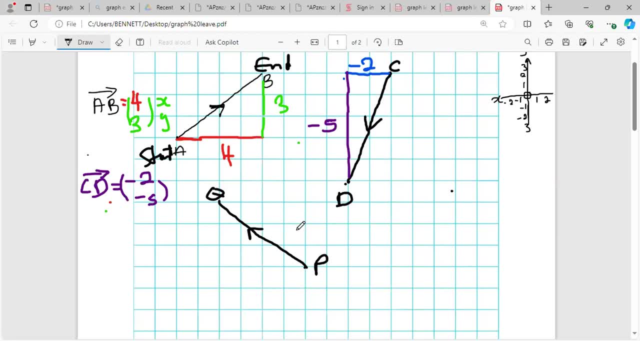 all right, let me call this pq. all right, what would call this one pq? let me ask guys, where is the endpoint on this? is it point p or point q? you know, sir, q5 and q, sir, yeah, because the arrow is pointing to words. yeah, it's pointing there. so it's only pointing towards the value of 3.324 h, right here. point for this up梅 trouble to the next up Kickstarter. montón for y taką is pointing at 0.325 h right of eg möe breakthrough. now we're nineteen, twenty, twenty40 h to fantastic. all right, you had some good players on the left hand side. in the left hand side. i'd like to ask you, um, if you can say anything, so just say what's the problem. you need to know. 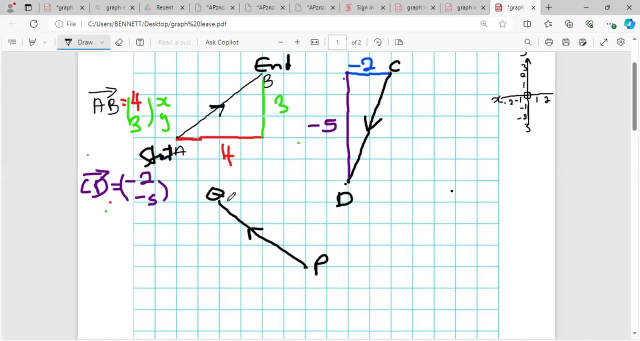 yeah, it's pointing towards q, so that mean we start at p, so you can just use your sentence. all right, you can't go up or down first. you have to either move left or right first. always x you have to do first, remember. you know, guys, nobody never teach me rectangle. i observe, my fellows observe this. 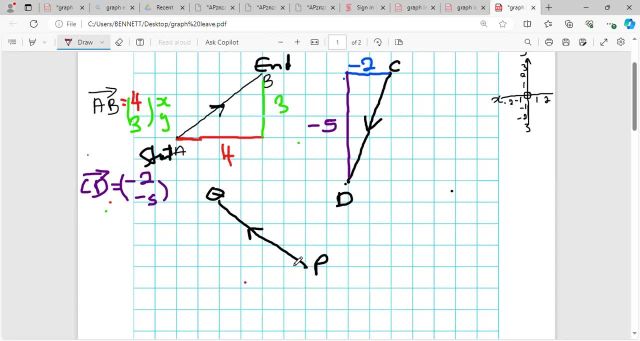 all right. this one when i talk to myself, talk myself, because when i was going to school, the teacher: they will never agree, cxc, never make it true, cxc, make a choose. so that means so we are going to be left first. so we have one, two, three, four. so that means it's negative four. 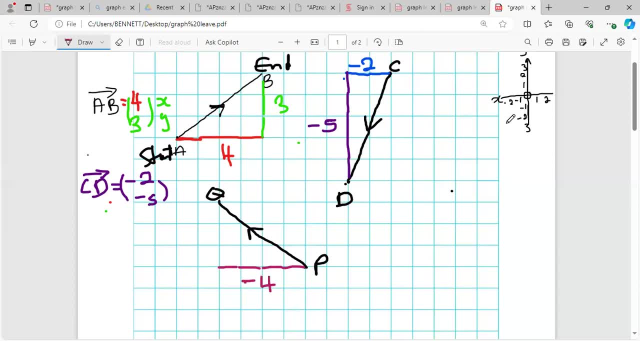 because once you go into your left, just like on the cartesian plane, x is negative, all right. and then now we're going up how we have to match it. you know we have to go straight to it: one, two, three. so this is: should this be negative or positive, or what you guys? 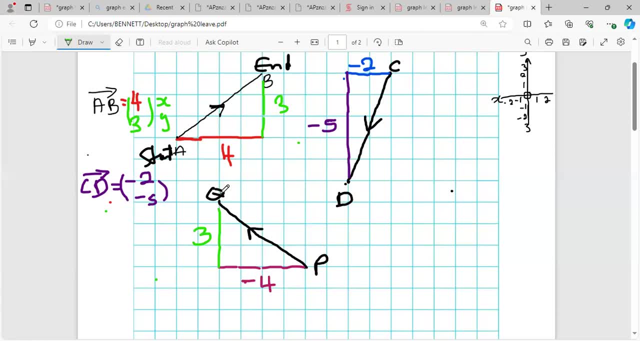 positive, sure, positive, because why you're going? oh, if this was a case where we're going down, then we would have negative three. but because we're going up, y has to be positive. so what we can do, you can just write from p to q. that's what it means. p is starting point. 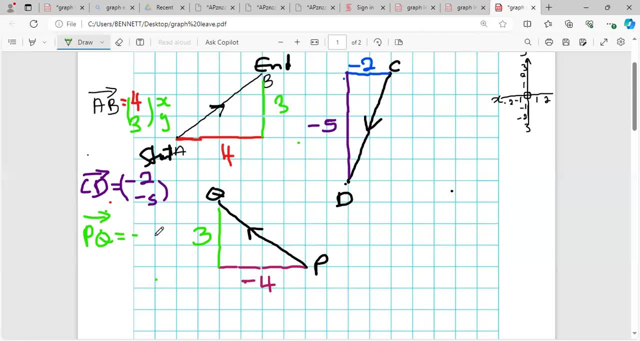 it's. i always do your x first, just like in the alphabet. so it's negative: four, three sir. yeah, man, go ahead. why you couldn't go up with from the p, why you couldn't go up all right? because you always have to move your x first. that's the rule. all right, always. 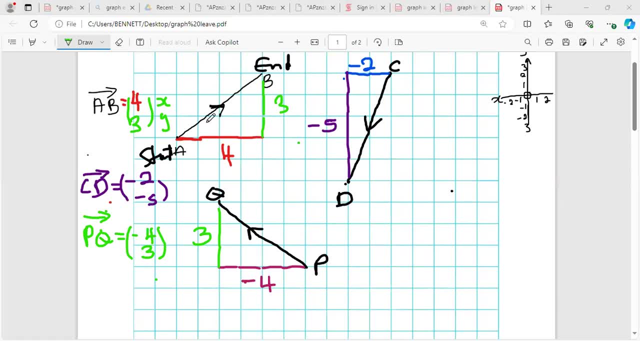 always cases just like with this. we start here, we could have easily go up, so right, no, we can't do that, always have to go because it's an alternate route you have to take. you know, with vector it don't go directly, so you just have to look where the starting point is relative to the end. 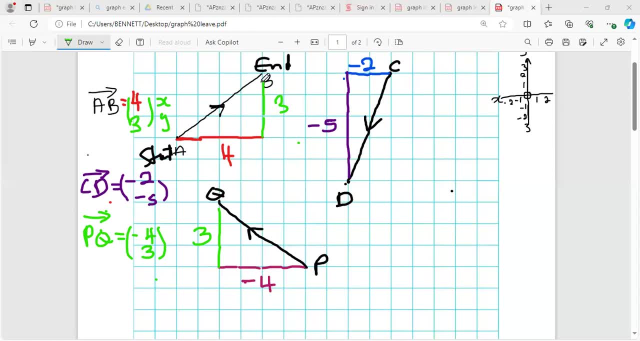 point, all right. so make a look at this scenario. we have, um, we have x positive, x, y positive, this negative, that negative. so x negative, y positive. that mean- i need to show you one nowhere- where x is positive and y is negative. that's the four scenarios that you can have, all right, 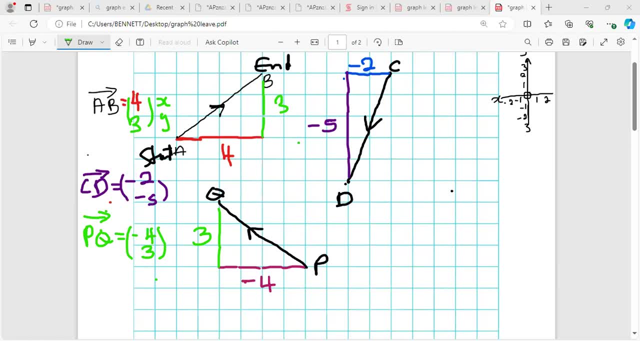 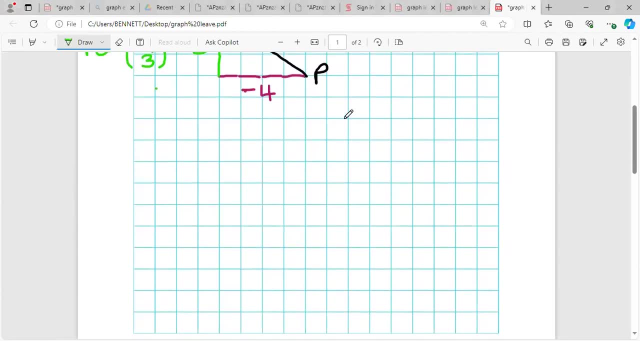 so of course you have one funny clip: more space. you know, guys, you have more speed. for this you would use a t graph. no, man, they don't necessarily have to give you a graph. you know, this is just to show you how vectors work. um, if it's, if, it's, if, if you're gonna need graph, if, normally after the position vector. 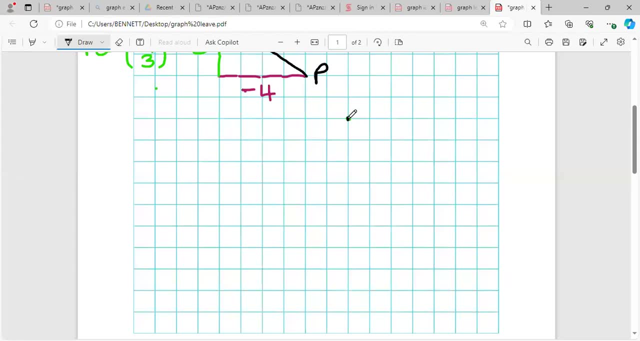 well, you see, once you understand how vector work, then it becomes so much easier for you. all right, let me use x and y this time. all right? so that's the x, that's the y, right, and, as i say, it depends on the starting point. this is the start, this is the end. whichever the error is pointing on, that's our endpoint. 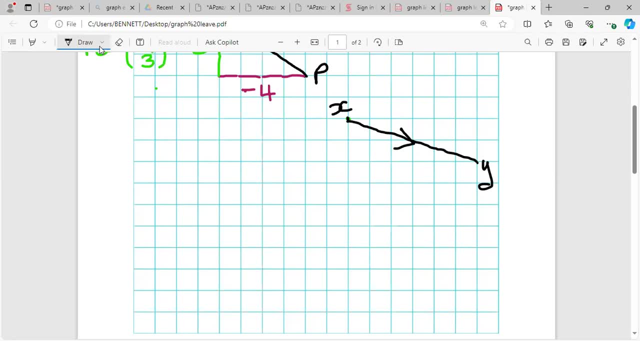 so to find the vector, what we need to do is we're going to start going to all right, because we cannot go so first, always either to our left or right. so we have one, two, three, four, five, six. now is this positive or negative? we're going to all right, positive, positive. thanks, anthony. 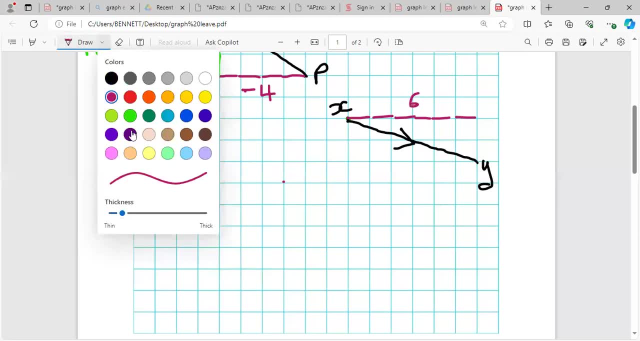 yeah, and then now to match it back, we're going down. so it's one negative negative. that will be negative, sir. yeah, that is it. so to write the vector now, it would be x, y, this over it means the vector from x to y. that is equal to six negative two, because you always have to write. 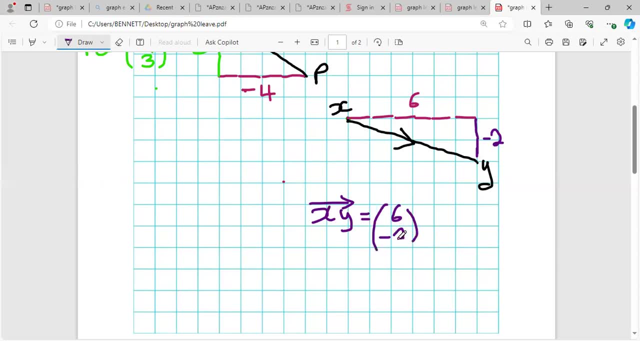 the x first guy. i think once you remember that, then you will. you cannot get it wrong. so the vector you can't find, yeah, man, go ahead. you can't get it wrong, so the vector you can't find you can't find. yeah, man, go ahead. you can find the vector of um, something on a plain paper. 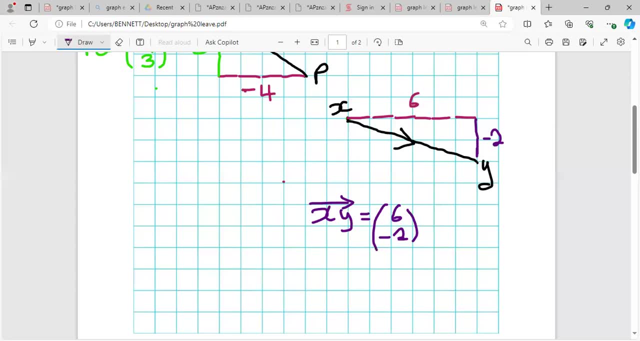 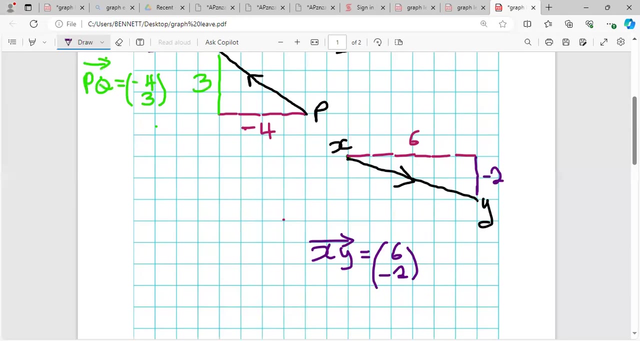 yeah, we can use algebra and find it to you know, but even if you have a plain paper, you can draw, you can draw it, but they will give you the, the coordinates, if they're gonna ask if you find the vector. but they make it easy for you, they will give you eternal grid. but if you have a plain, 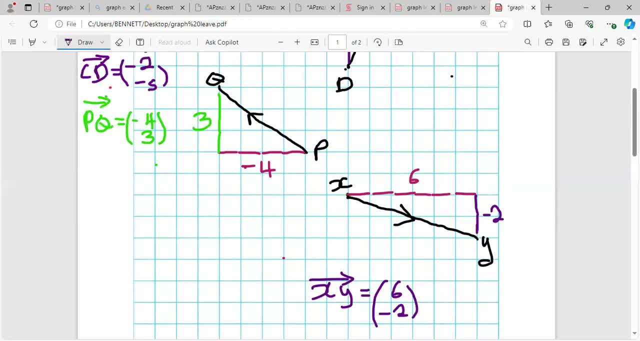 paper. you can be r. if it's a position vector, they will. they will um, give you the coordinates and so. so the only difference with this guys notice, there's no number and degree, but yet we can create the numbers and the position vector. we actually use the contagion, in a sense because 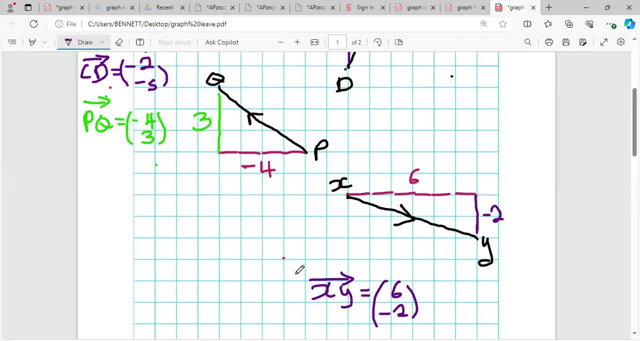 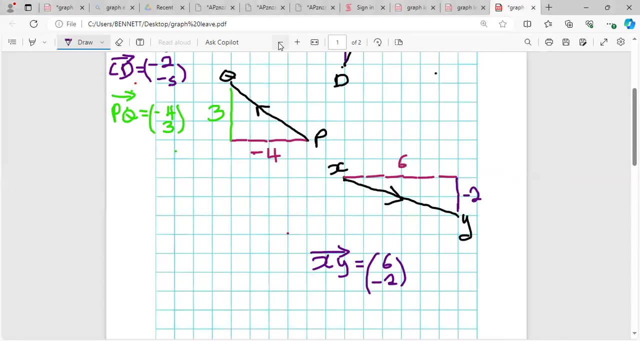 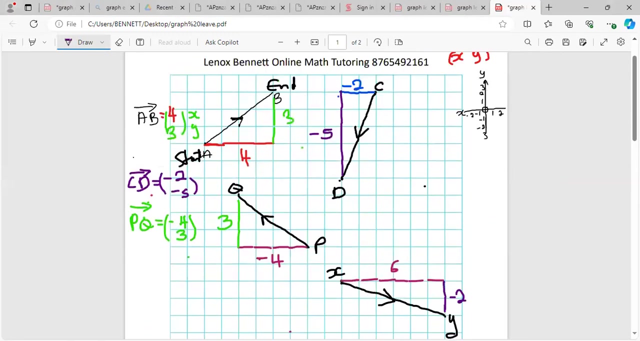 they start at the point zero, zero. somebody are playing music, man. all right, that would be easier. So I'm going to look at all four scenarios, because this is basically. it can be different from this. It's either one of them. here, it's either two positive, two negative or X negative. 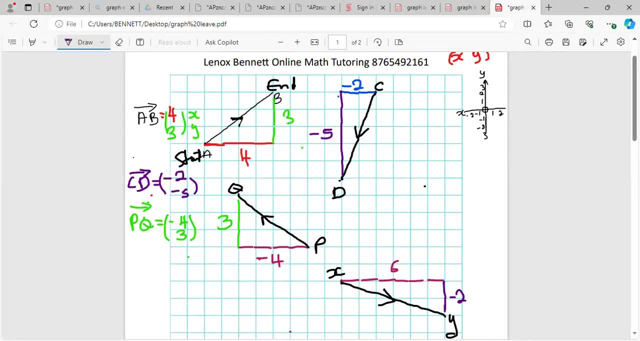 Y positive, or Y positive, X negative. This is just the four scenarios that you can have. So, sir, when I'm asking, so right a vector, sir you're going to get like, so let me. 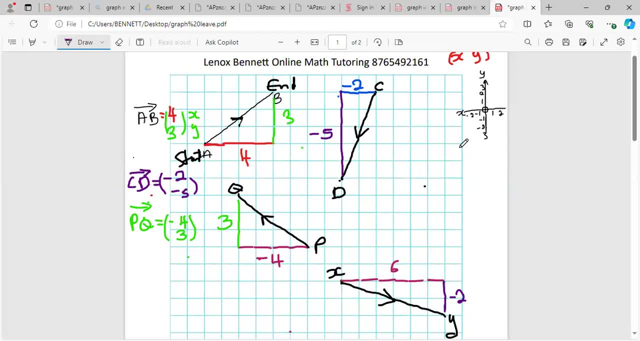 see a T-graph on the right from the screen. that's why I'm going to ask if that's in the value. Well, you see, this was just to explain, when you go into our left and to our right, Why, when we go into our left, it's negative on the X. 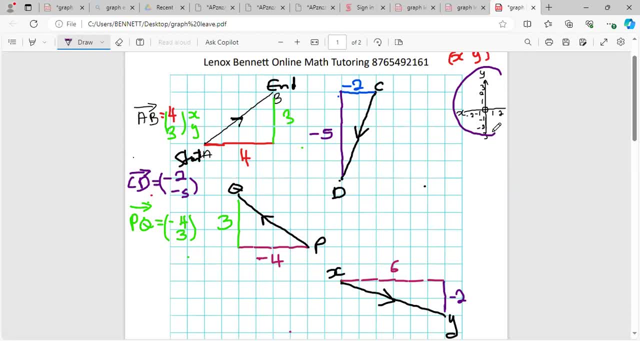 Why, when you go into our right, it's positive because it's based on the Cartesian plane. All right, sir, thanks, Yeah, Yeah, I think Because I came in a little bit late that was, But this is what we're reasoning, right. 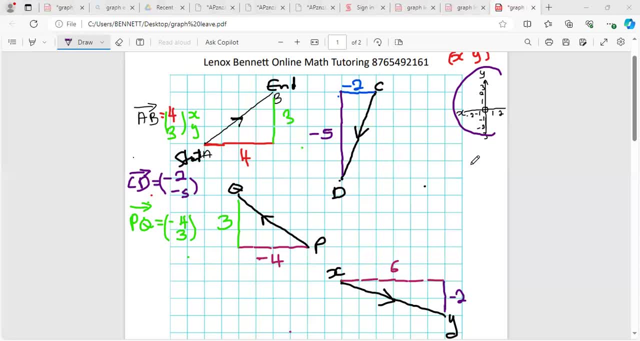 So that's all you know, All right. So any questions? Sir, can I pull up the screen a little? You guys have your graph leaf. Wait, let me just. You guys have graph leaf, because I requested that you guys have graph leaf. comes on there. 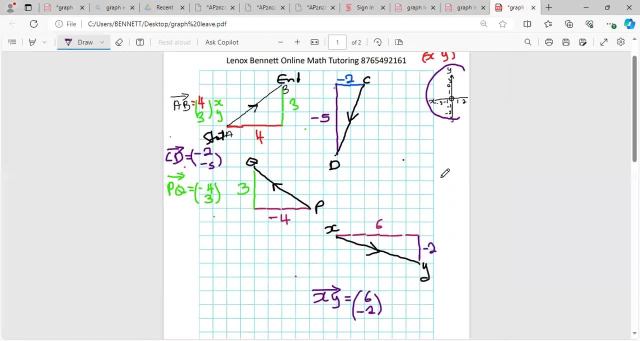 If you do, you can take it out, please, Just to see if where we are. Yes, sir, I will give you. Yeah, And guys, you can take your time and draw it as neat as possible. We just want to get this thing on the way. 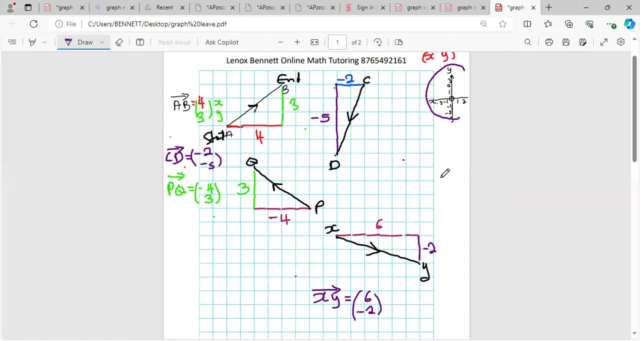 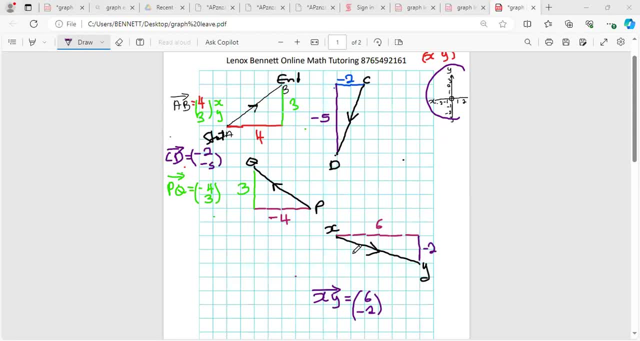 I don't see anybody. Oh, Oh yeah. Oh, you're on, Shania. I just got to take cinema. I just seen it. Shania, you're 20 minutes late, man. Oh God, Oh God. 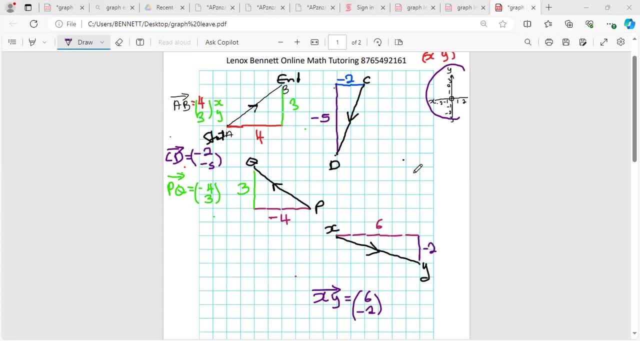 Oh man, I'm doing it. Alright, Shania, I'm partying, Nevermind You here, you have to score as many as you want. I am. I don't know what I'm doing. Yeah, this is. 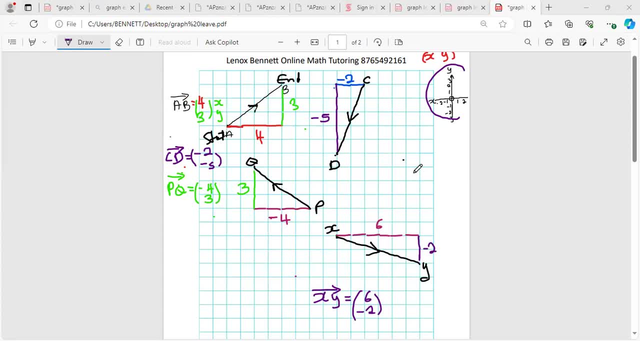 I was speaking for. Thank you so much. Thank you, Yeah, You're welcome. So just Yes, no problem, gorgoffclawcom, Thank you so much. No, no problem, Forget it, Lenny, You're получается. 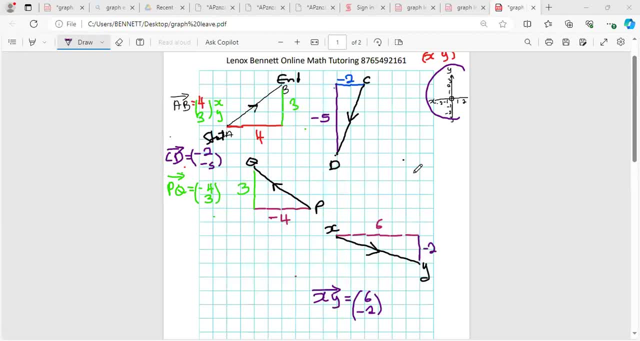 Oh, for the new person. yeah, with your name here, I just become expecting unity in the person. all right, guys. so please ensure that you have these examples and if you have any questions, before we attempt for you guys to try some on your own. so now in Wednesday, hopefully everybody can see the content. as I said, guys, it 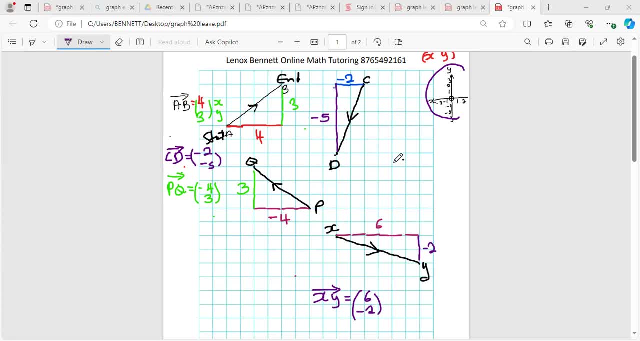 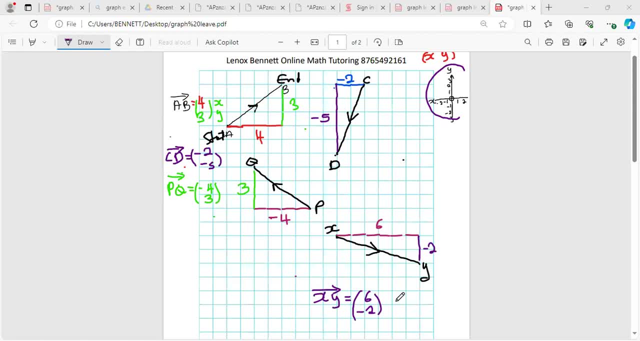 oh, all right, guys, do them meet here. I'm positive, do them meet as possible, because I really want you guys to um.